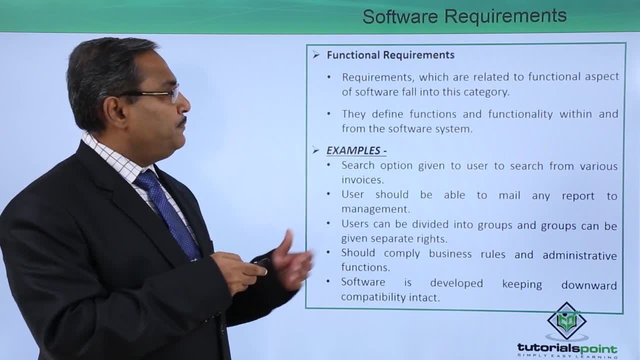 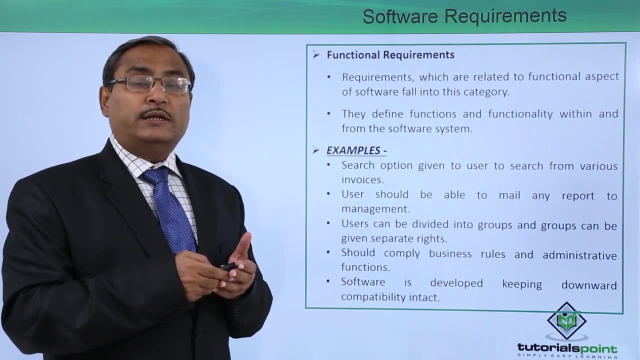 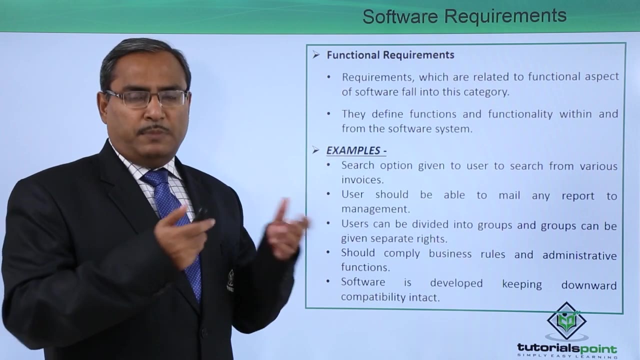 So what is the? what are the functional requirements? So requirements which are related to functional aspect of the software fall in this category. So what is? the functional requirements are getting implemented. So let us suppose, say, one transaction may be treated as a functional requirement. 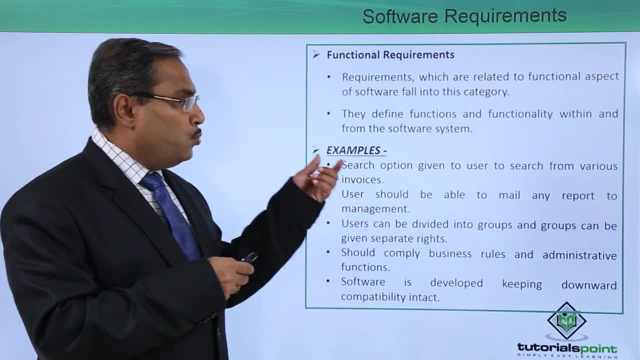 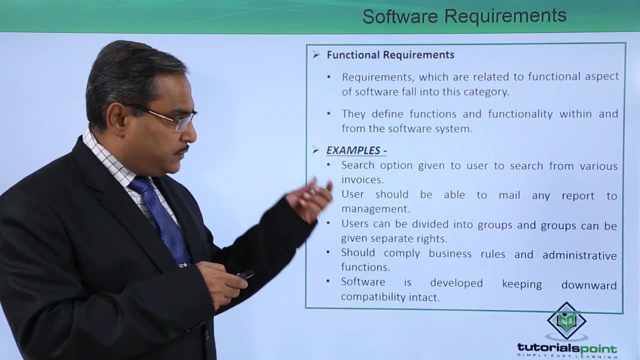 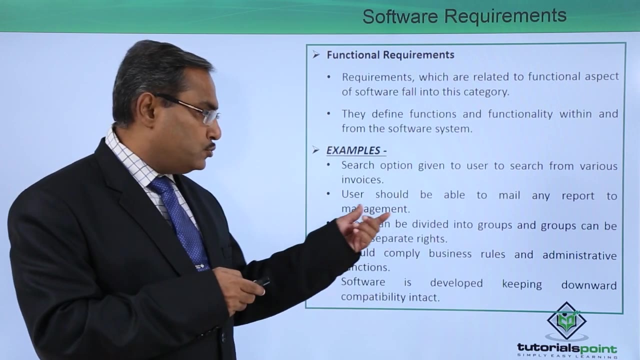 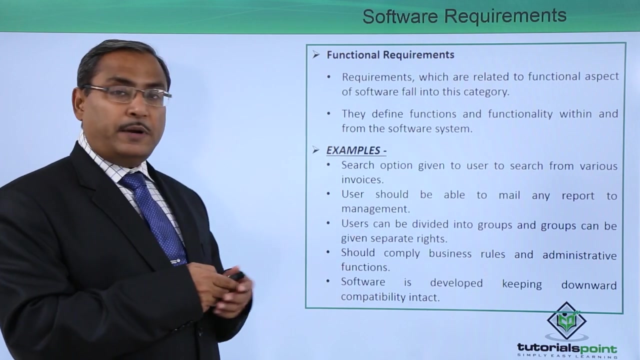 So they define functions and functionality within and from the software system. So examples: so search option given to user to search from various invoices. so this is a functional requirement. User should be able to mail any report to management. Users can be divided into groups and groups can be given separate rights. 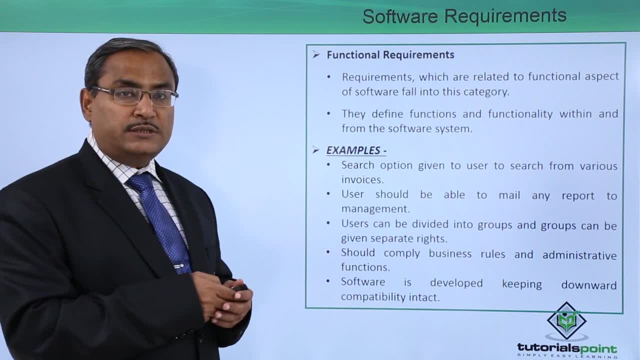 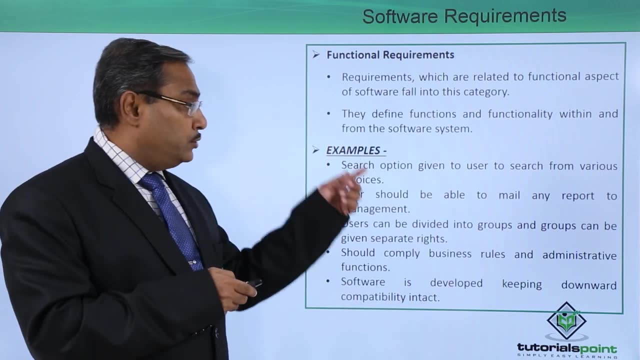 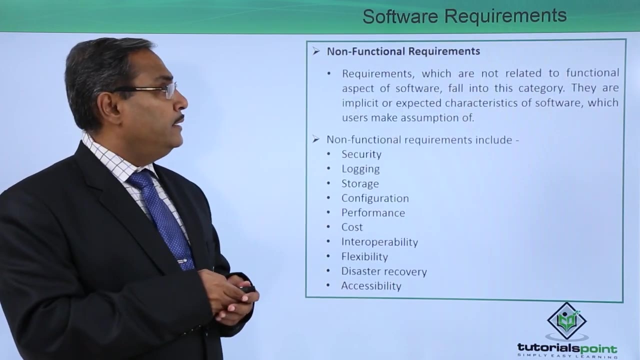 Should comply business rules and administrative function and software is developed keeping downward compatibility intact. So these are the different requirements which are coming under this functional requirements category. Next one we are going to discuss: there is a non-functional requirements, So requirements which are non-functional. 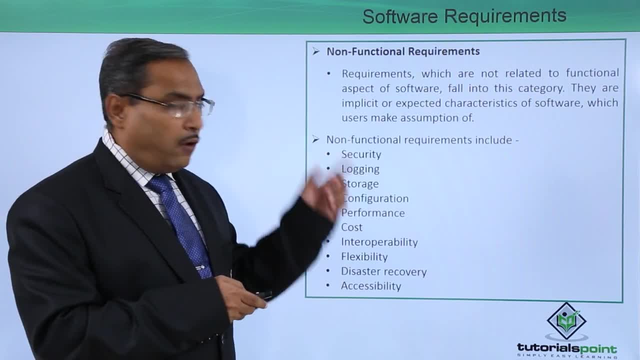 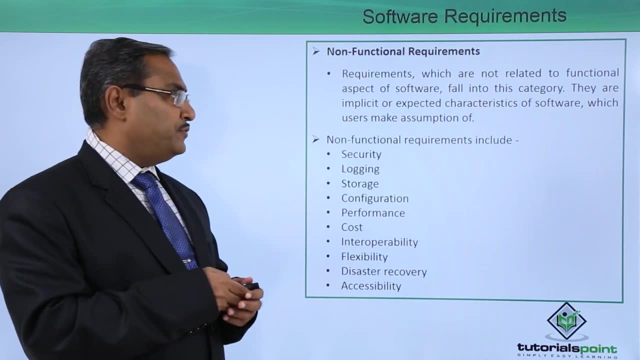 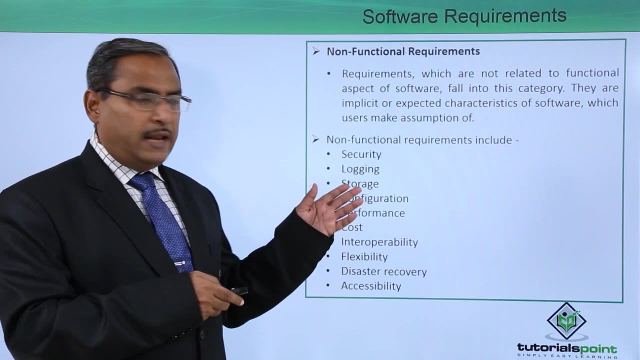 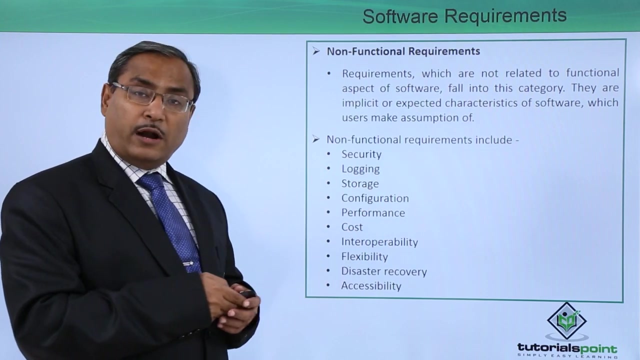 So not related to functional aspect of the software, will fall in this respective category. They are implicit or expected characteristics of the software which user make assumption of. So some of the non-functional requirements might be like this: So security, logging, storage, configuration, performance, cost, interoperability, flexibility. 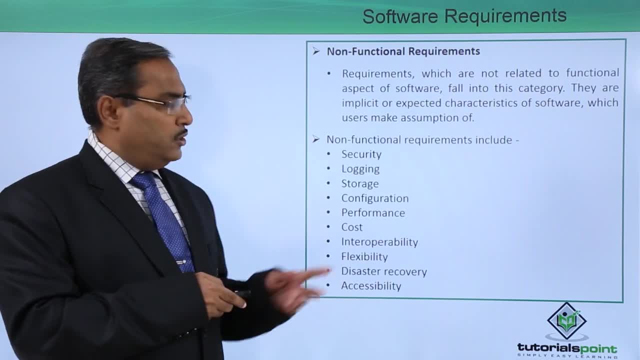 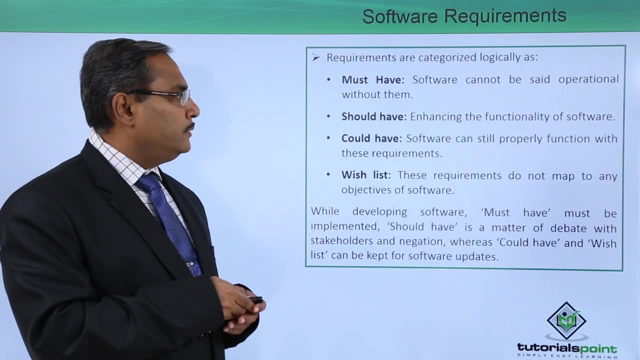 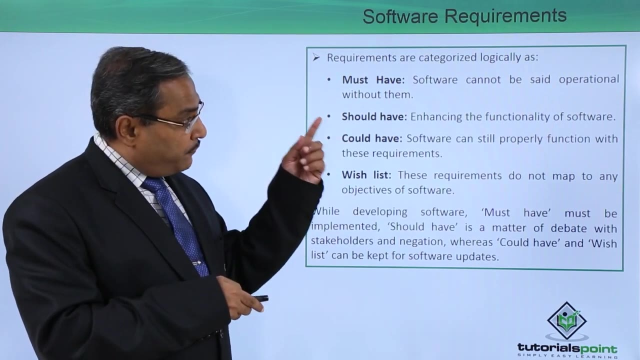 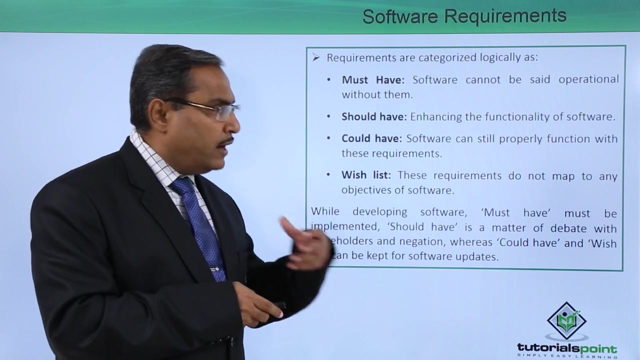 disaster recovery, accessibility. So all these requirements are falling under the non-functional requirement category. Recommends are categorized logically as must have, that is, a software cannot be said operational without them, So must have requirements, should have enhancing the functionality of the software. that means 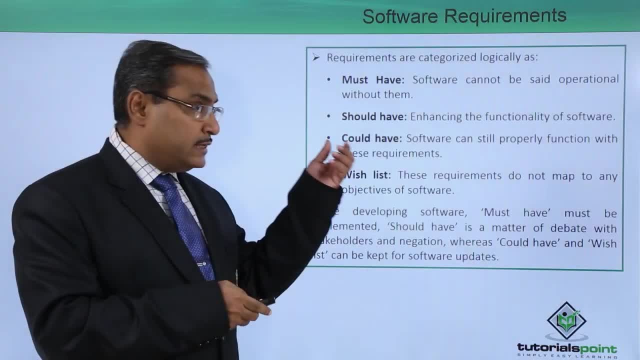 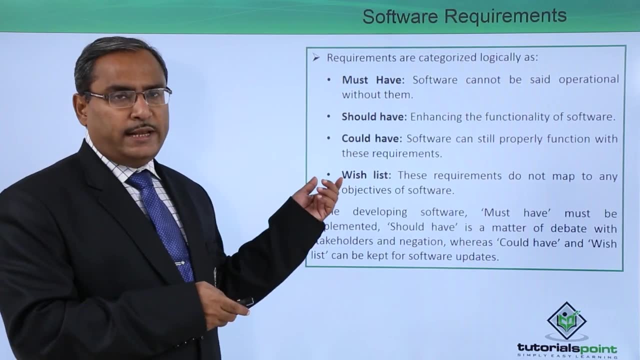 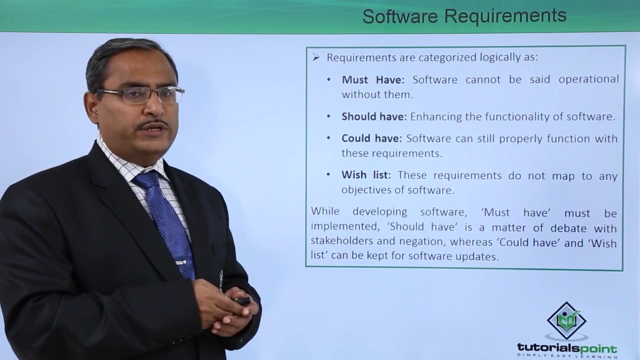 it is preferred to have those requirements, So software can still properly function with these requirements. That is coming under this could have. Next one is the wish list. So these requirements do not map to any objective of the software, but it is in our wish list.